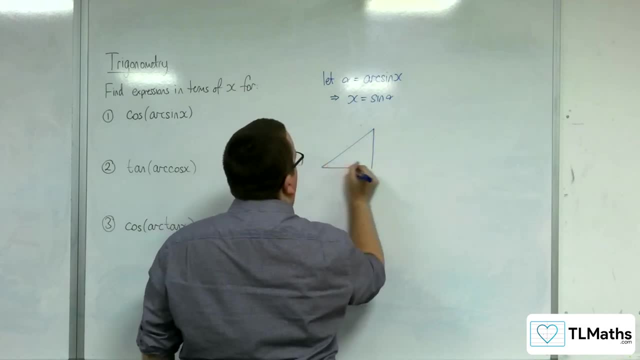 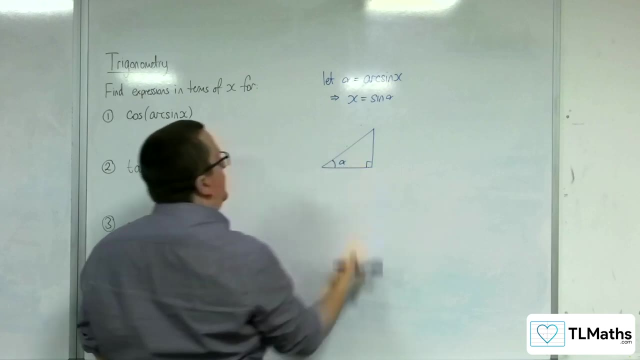 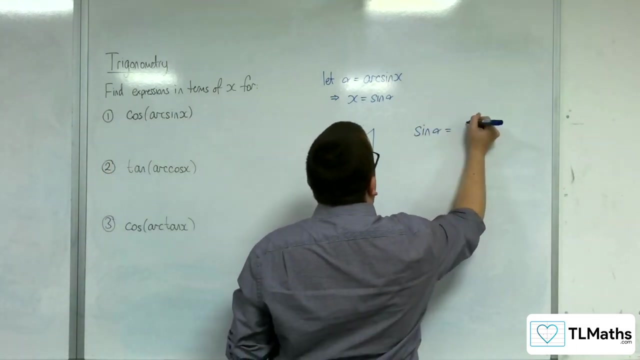 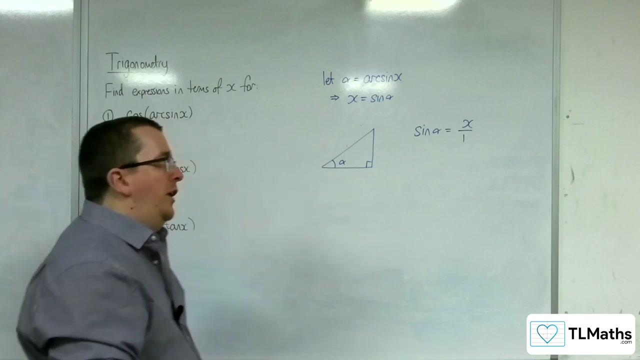 Now if I draw a right angle triangle, OK, here is my angle alpha. Now if I'm saying that sine of alpha is equal to x, OK, I could also write the x as x over 1.. Now I understand that with SOHCAHTOA sine is opposite over hypotenuse. 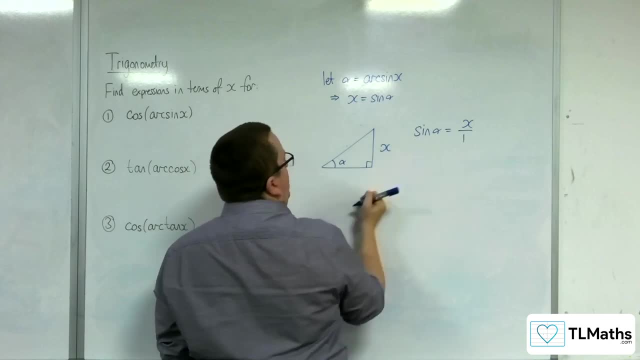 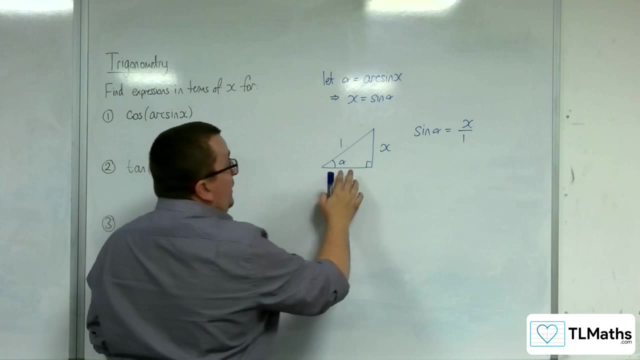 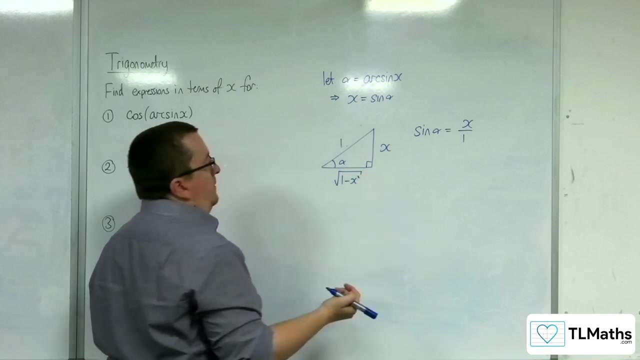 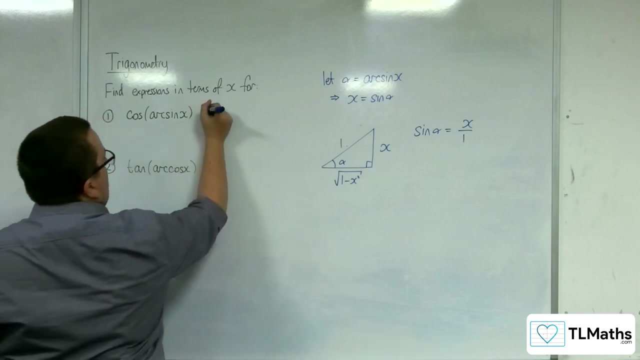 So that means that if that's the opposite side, that is x, and the hypotenuse must therefore be 1.. So the missing side that we have here is the square root of 1 minus x squared using Pythagoras. So if I'm looking for cosine of arc sine x, this is cosine of alpha. 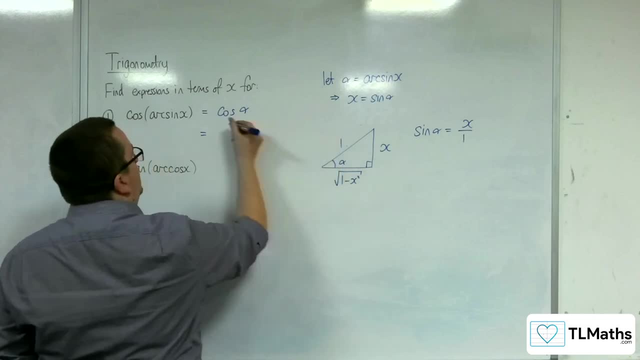 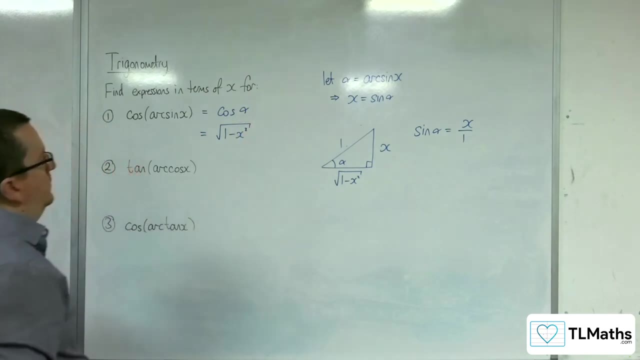 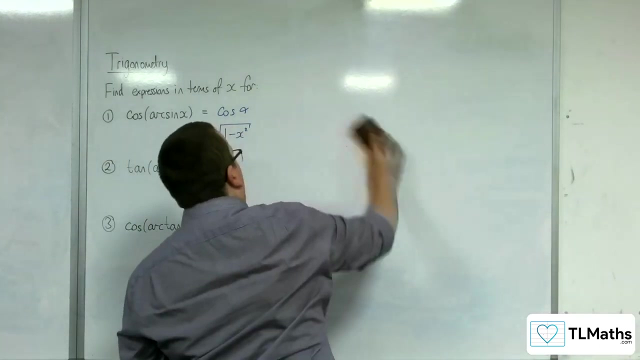 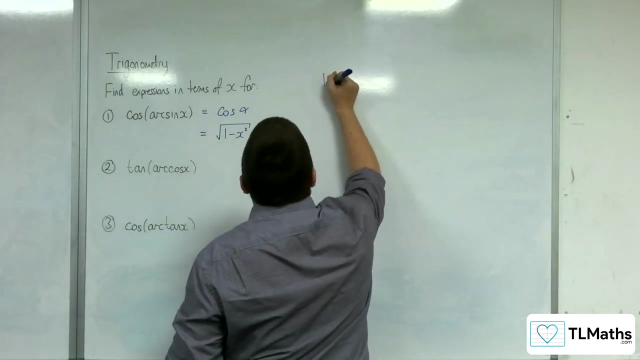 Cosine of alpha is the adjacent over the hypotenuse, And so we get the square root of 1 minus x squared Right. so we're going to use a similar method for these others. So tan of arc cosine x. So let's say beta is arc cosine of x. 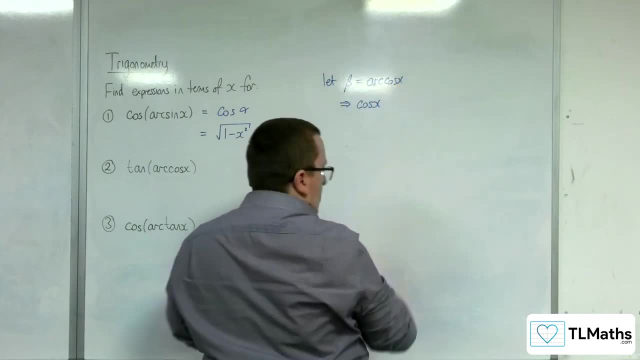 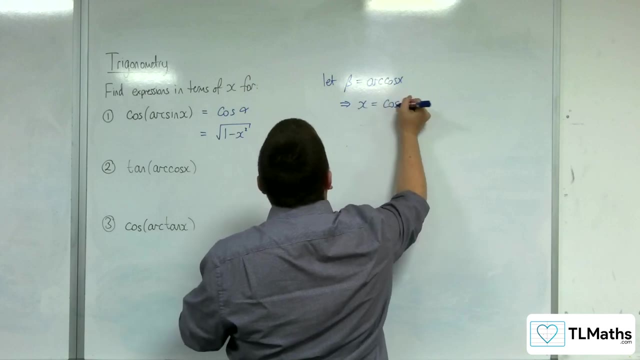 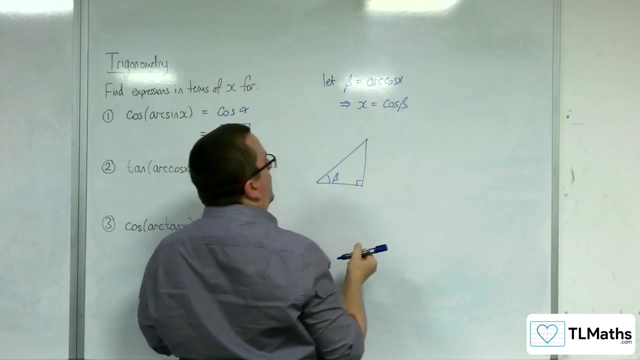 So that means that cosine of x- oh, sorry that x, rather this way, that x- is cosine of beta. Right, let's draw a right angle triangle. There's my angle beta. So if cosine of x is cosine of beta, then that means that x is cosine of beta. 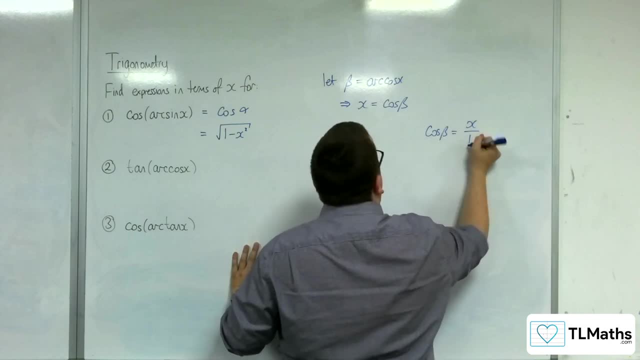 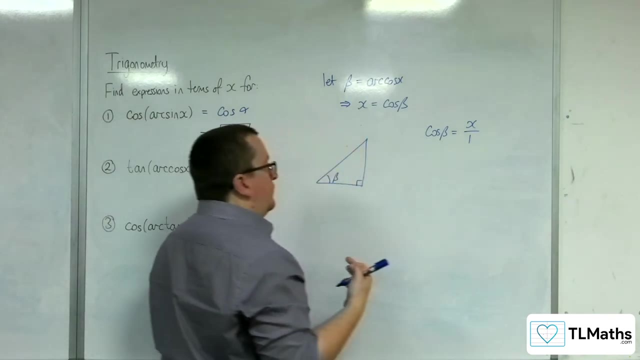 If cosine beta is equal to x, we can write that as x over 1.. We know that cosine using Sokoto is adjacent over hypotenuse. So if the adjacent side is x, the hypotenuse is 1, then the missing side is 1 minus x squared, square rooted. 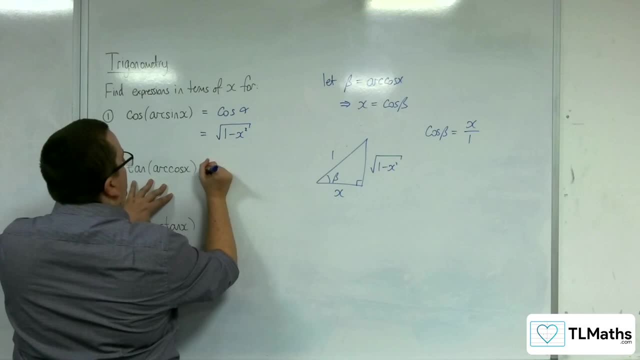 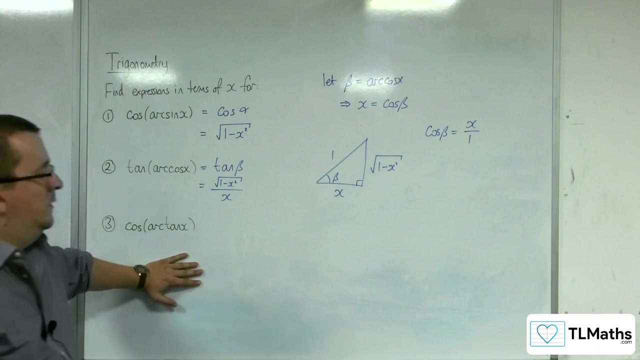 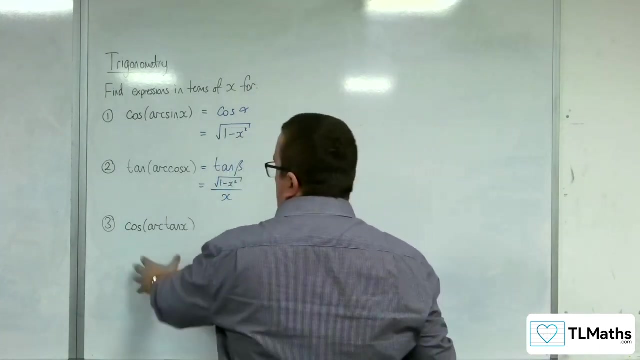 So if I'm looking at tan of arc, cosine x, this is tan of beta, Which is equal to the opposite over the adjacent. So that's the square root of 1 minus x squared over x. Okay, So number 3, cosine of arc tan x.